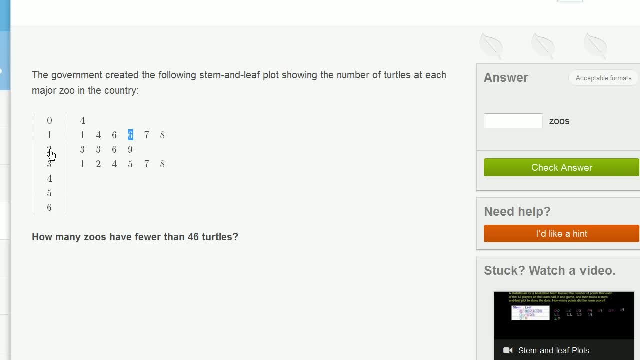 All of this. this is 23.. This is 23.. This is 26,, because we have our tens place right over here. This is the first digit, So let's go answer the question: How many zoos had fewer than 46 turtles? 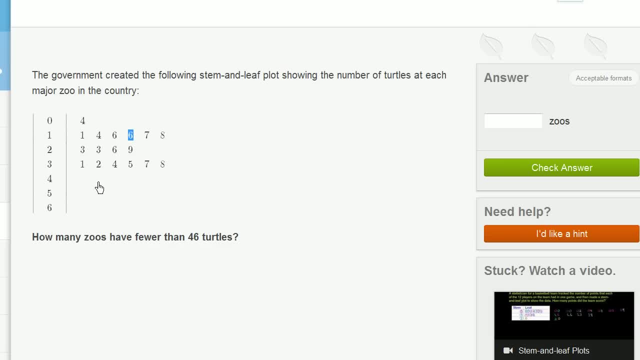 So there are no zoos that had 40 anything turtles, And so all of these zoos here. so all of these had 36.. These had 20 something turtles. These had 20 something turtles. These have in the teens. these have single digits. 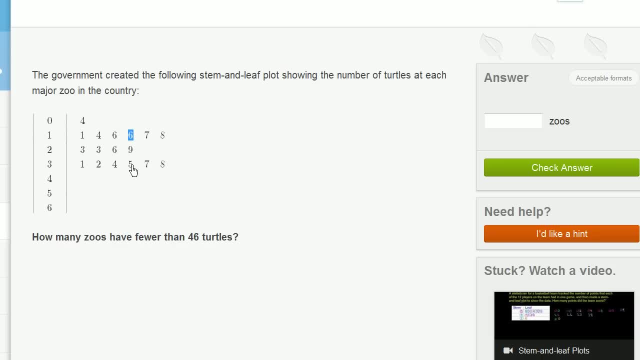 So it's literally as many zoos as we have listed here, So 1,, 2,, 3,, 4,, 5, 6,, 7,, 8,, 9,, 10,, 11,, 12,, 13,, 14,, 15,, 16,, 17.. 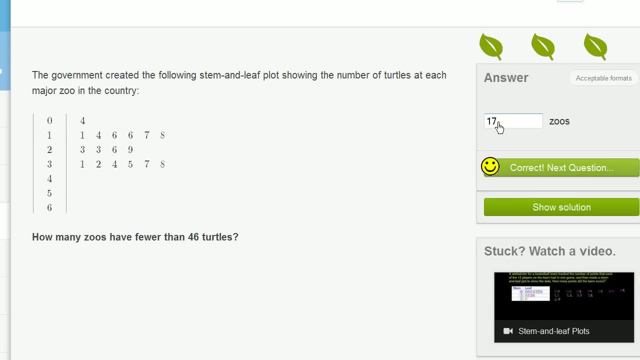 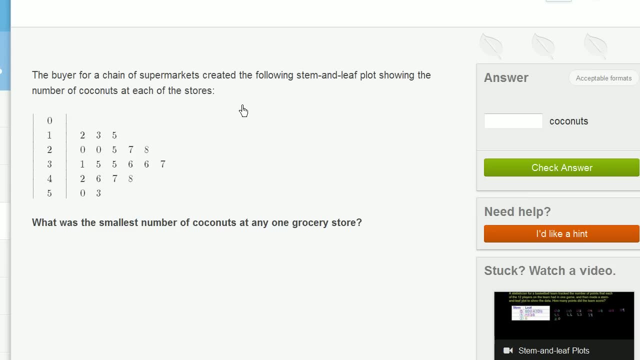 17 zoos have fewer than 46 turtles. Let's do another one. The buyer for a chain of supermarkets created the following stem and leaf plot showing the number of coconuts at each of the stores: What was the smallest number of coconuts? 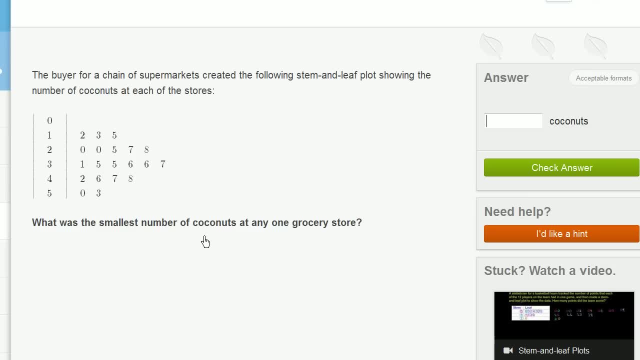 at any one grocery store. So the buyer for a chain of supermarkets created the following stem of leaf plots showing the number of coconuts at each of the stores. So, at any one grocery store, the smallest number. well, that's this one right over here. 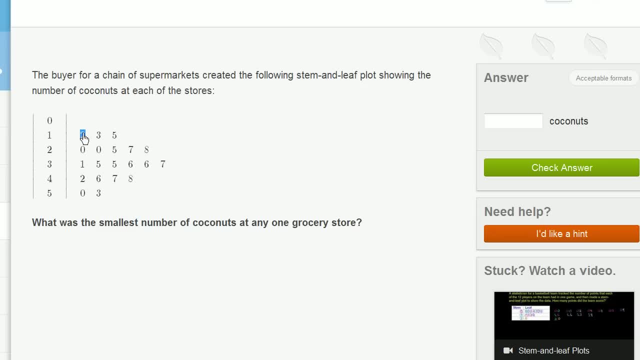 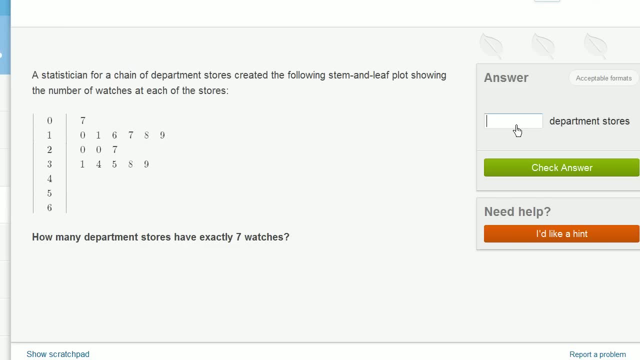 And remember it's not 2.. We have our tens places right over here. It's a 1.. So this right over here represents 12 coconuts at that store. So we'll put 12 right over here. Let's try it on another one. 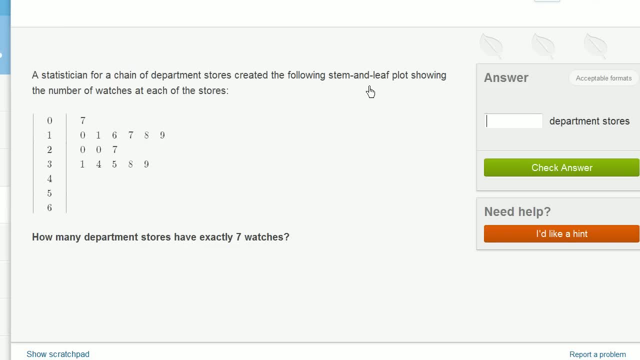 A statistician for a chain of department stores created the following stem and leaf plot showing the number of watches at each of the stores. How many department stores have exactly 7 watches? Well, that's only this one right over here: 0, 7 watches. 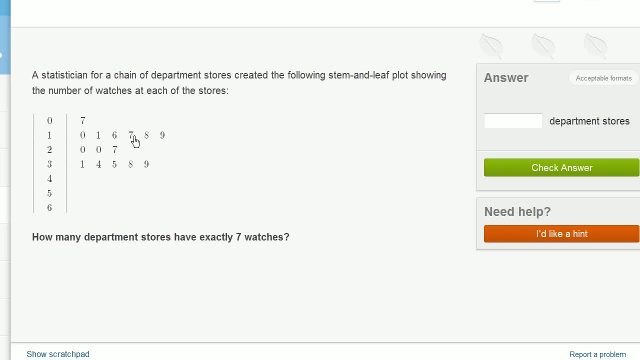 This one right, this, this and that one are not 7.. This is representing 17 because it's in the row with 1 at the beginning. This right over here represents 27 because it's in the row with the 2 at the beginning. 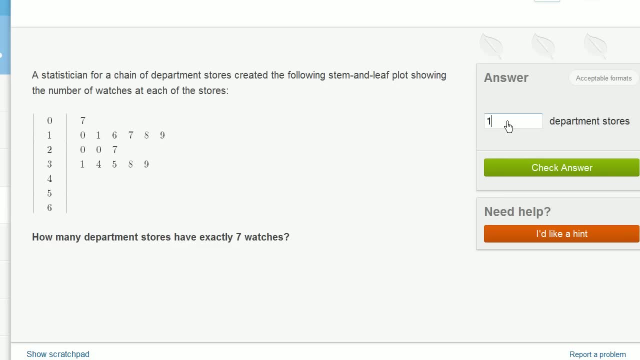 So there's only one store that has exactly 7 watches. Let's do one more. This is kind of fun. A zookeeper created the following stem and leaf plot showing the number of tigers at each major zoo in the country. How many zoos have more than 24 tigers? 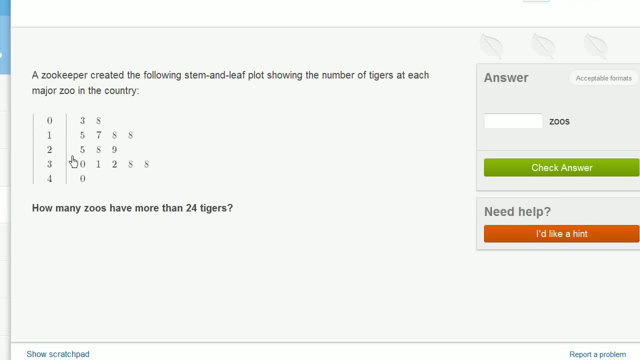 So we could ignore the 0s and the teens And we get into the 20s. This is 25.. So that meets the criteria. And then you go to 28,, 29.. So all of these, all of these in the 30s,